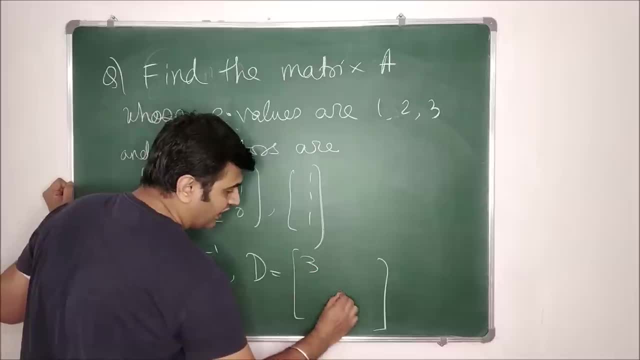 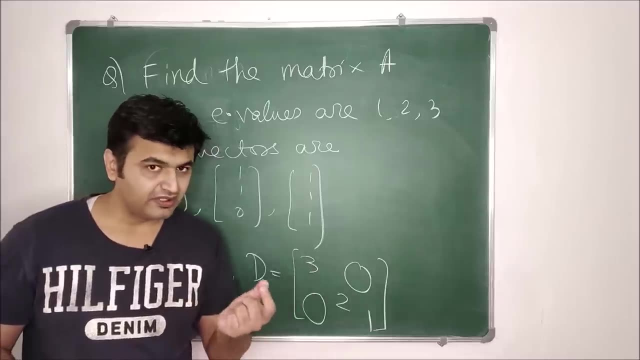 are nothing but the eigenvalues. So eigenvalues are 1,, 2,, 3, I usually keep, I will usually write in the design descending order, because the highest eigenvalue are of pretty much different. I mean, if you study data science or machine learning in future, then you will. 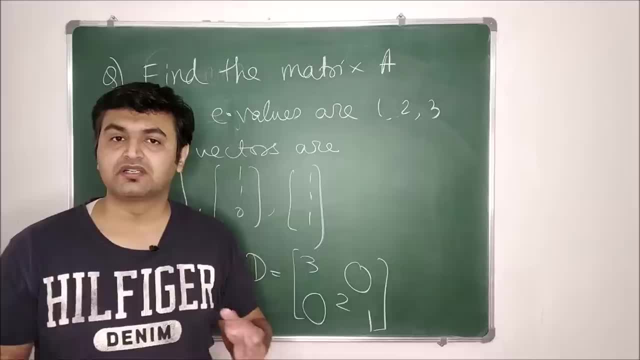 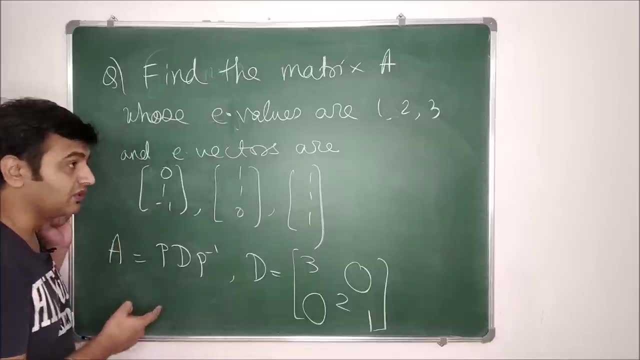 see that highest and the smallest, these two eigenvalues, usually play a larger role. Okay, so let somebody is this. Okay. now question is: first of all, is your matrix a diagonalizable? That means whether you can write A as this decomposition. Answer is yes, Why? Because? 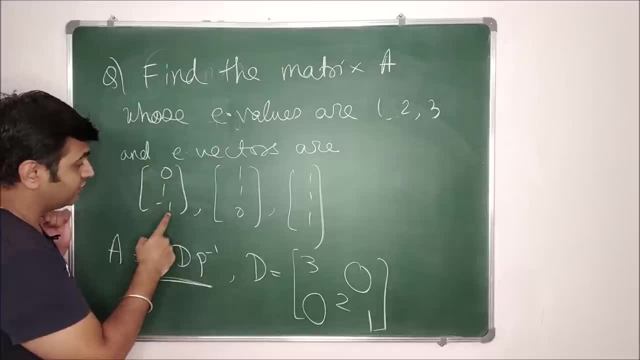 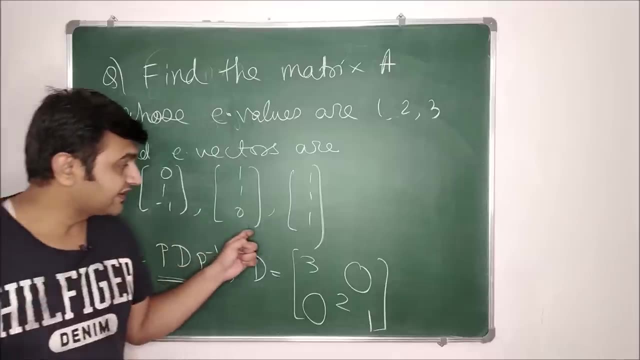 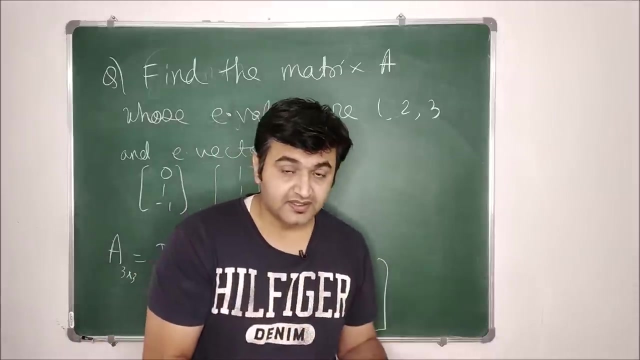 A is a matrix of order three cross three because, as you can see, the vectors of order three cross one. So this is three cross three And, as you can see, these three vectors are linearly independent. Why so? Because, if you recall a nice theorem from linear algebra, eigenvectors corresponding. 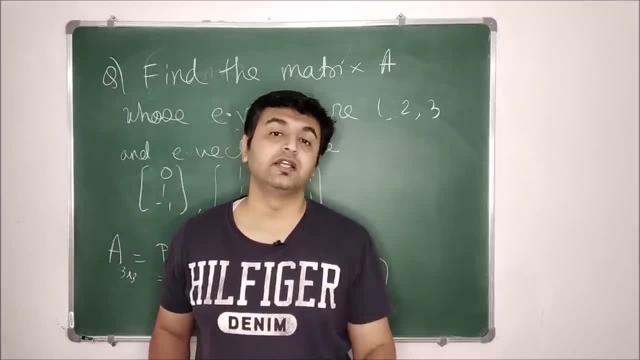 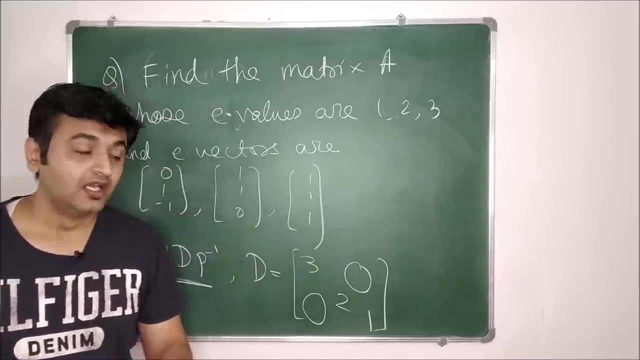 to distinct eigenvalues are always linearly independent. So eigenvalues are distinct. Yes, Therefore the corresponding eigenvectors are linearly independent. So therefore, for a three cross three matrix, we are having three linearly independent eigenvectors And 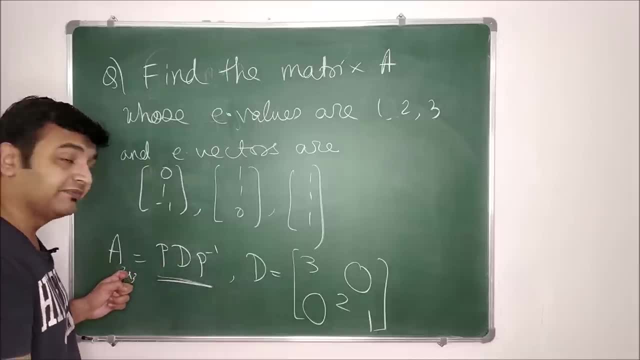 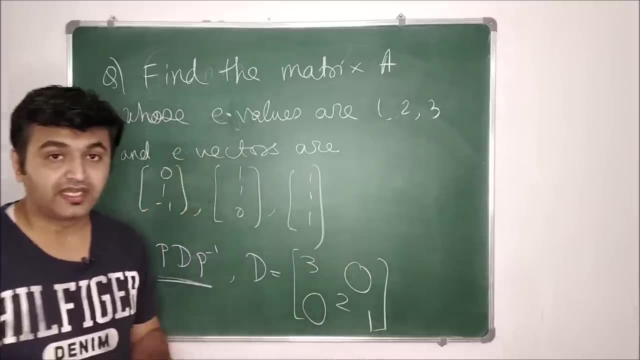 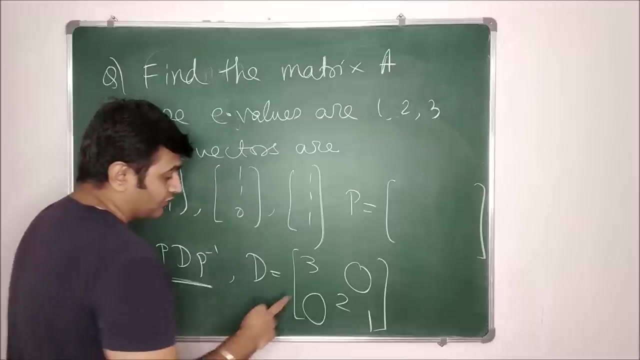 therefore the matrix is diagonalizable. That means A can be written as PDP inverse. So what is my D? it is a diagonal matrix whose diagonal entries are the eigenvalues. What is my matrix P? it is the matrix whose column vectors are the eigenvectors. So first I have written three over here. So first the eigenvector. 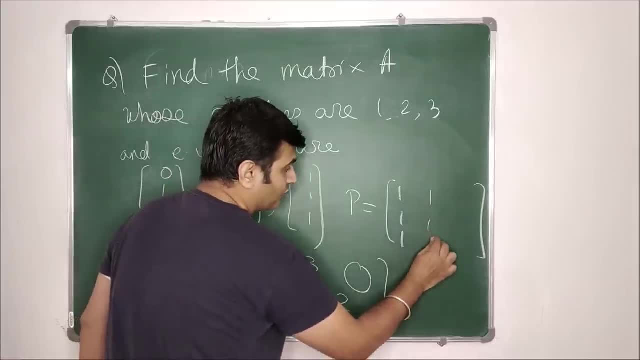 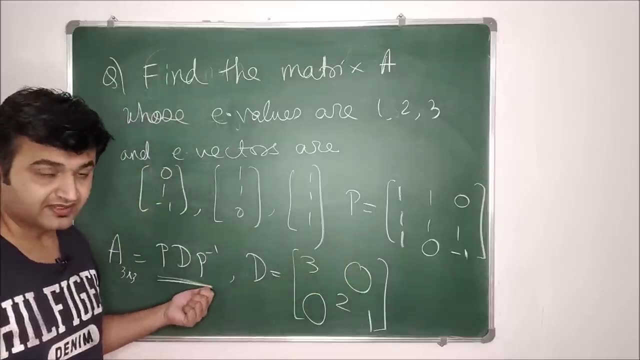 for three will come, then two, so then the eigenvector for two will come, and then one, so eigenvector. So this is my D, this is my P. Now, what is the next step? you need to find P inverse. 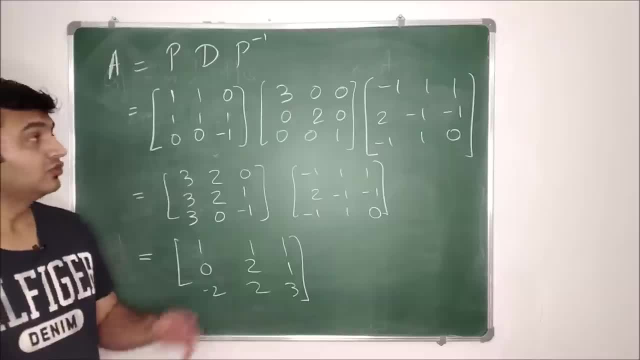 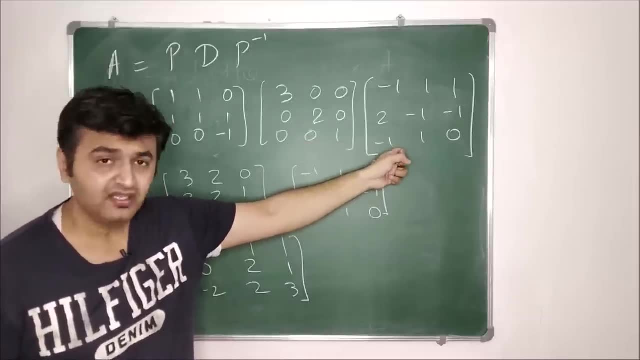 So I have calculated P inverse, So let me write it down directly. So our A is nothing but PDP inverse. So I wrote the matrix P, the matrix D and this is my P inverse. you can calculate and verify. Okay, so now. first I did this: two matrix multiplication, which 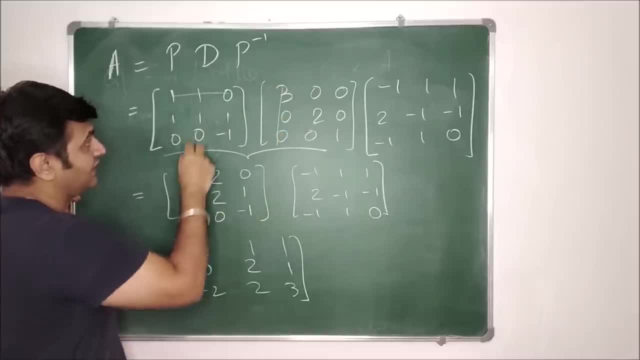 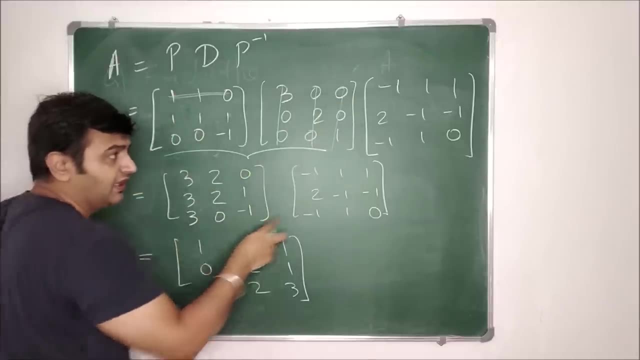 is this entry: 110 into 300 is 3,, 110 into 020 is 2,, 110 into 001 is 0.. So you do this multiplication and P inverse is as it is, And then you do this two multiplication And therefore: 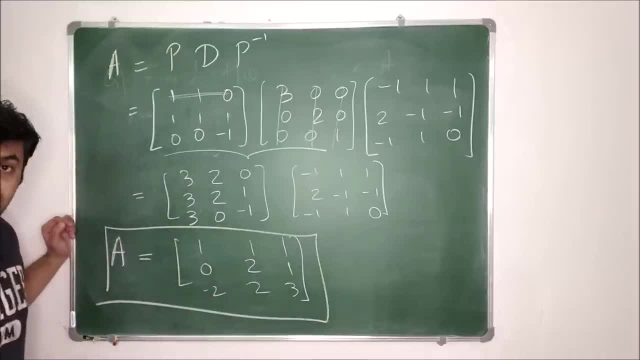 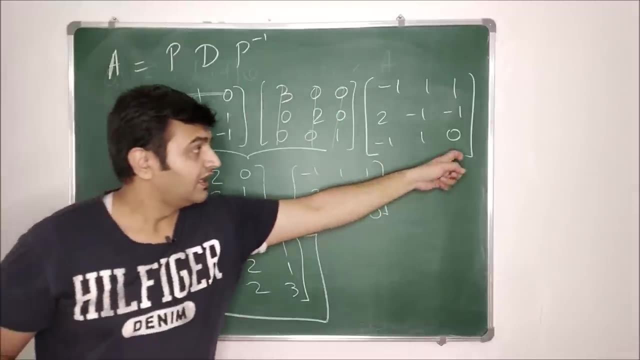 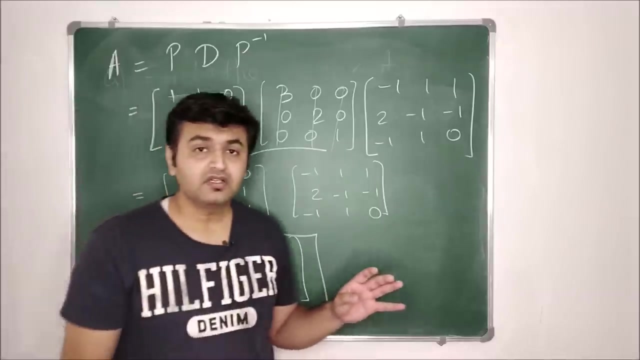 this is the required matrix A. You can check that. you can try to find eigenvalues and eigenvectors for this matrix. you will get the same answer: 123 as the eigenvalues and these three as the eigenvectors. So this is one of the very important steps. So whenever there's a question, 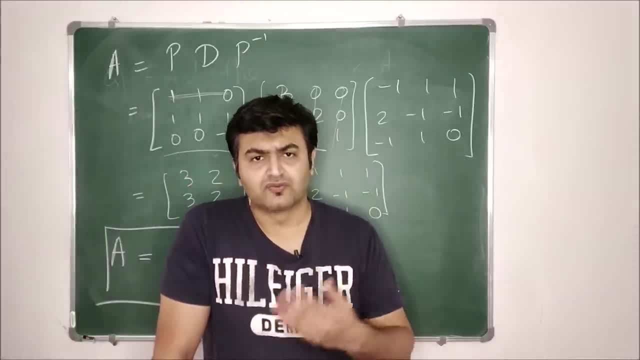 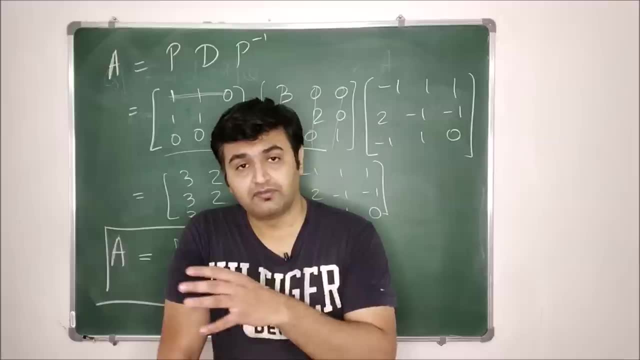 on finding the matrix of whatever order, say 4 cross 4,, 5 cross 4, you and so on. And it is in the question if it is given that these are the eigenvectors. So just see, if matrix is three cross three and three linearly independent eigenvectors are given. go by this way. If 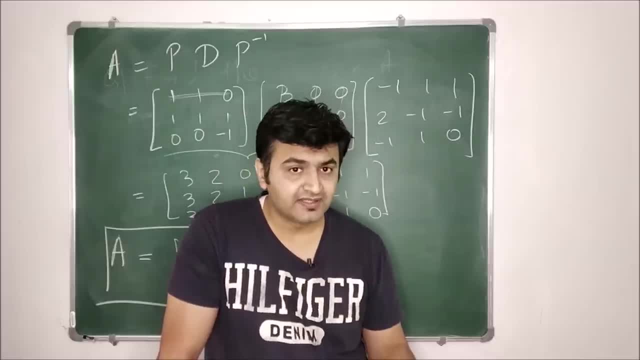 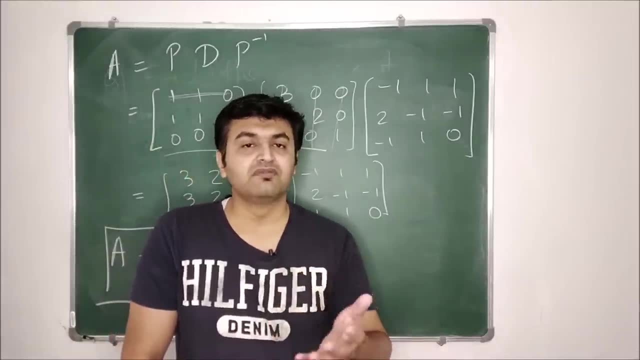 matrix is of order two cross two and two linearly independent Eigenvectors are given. good, you can apply this. Okay, so that's how one can solve this kind of problem. Now let me give you one homework question. So your job is to find the matrix. 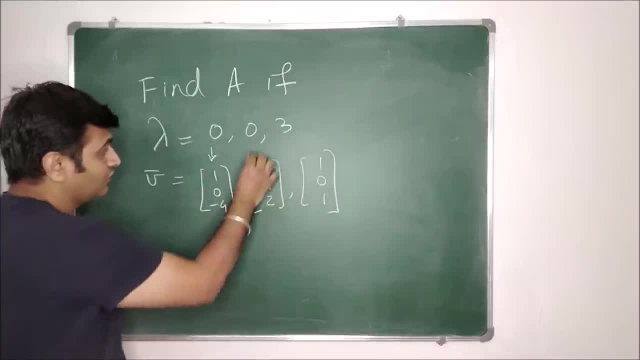 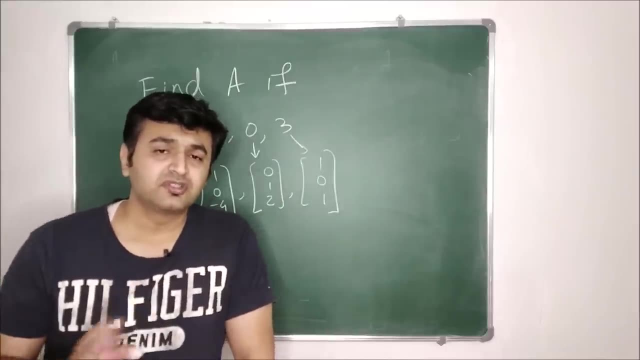 A eigenvalues are 003.. So for zero, these two are the eigenvectors and for three, this is the eigenvector. See, when the eigenvectors are distinct, you are not supposed to worry about them. So when the eigenvectors are distinct, you are not supposed to worry about them. So 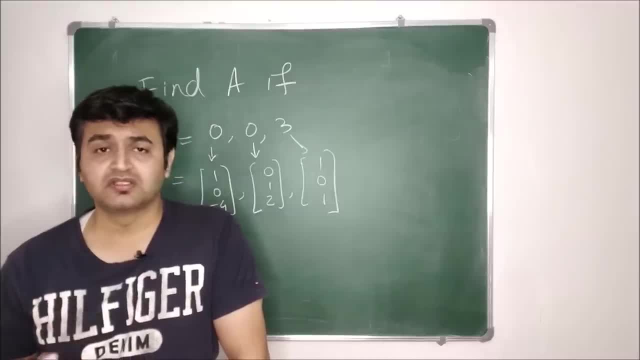 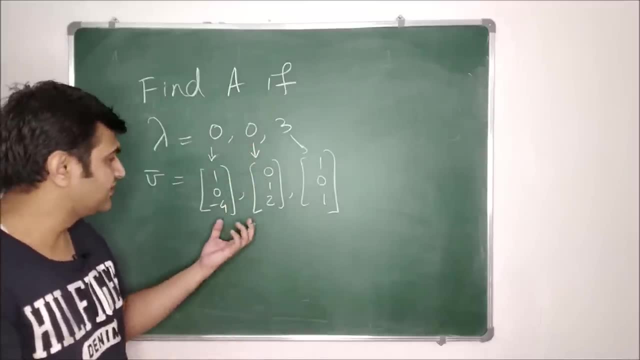 So in the case of zero, this is the eigenvector. So for three, this is the eigenvector. So about the eigenvectors: because eigenvectors are linearly independent for distinct eigenvalues, For repeated eigenvalues- now they have mentioned too- that means it has to be obvious that these 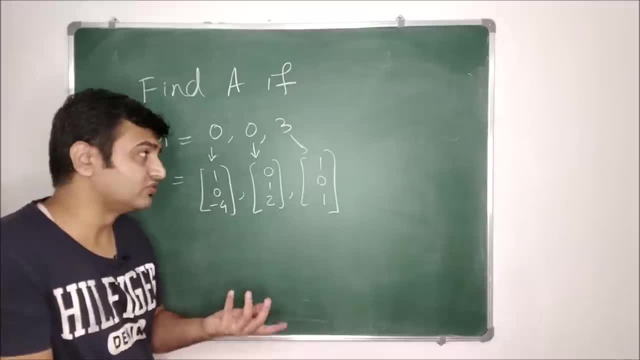 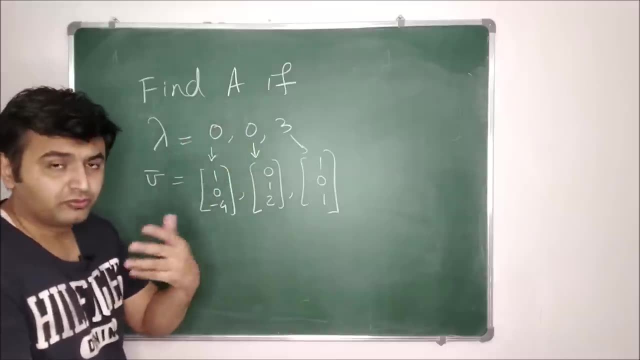 two are independent. but just for safer side you can cross check also because for here algebraic multiplicity is 2, so geometric multiplicity has to be 2 for the matrix to be diagonalizable. that means for the matrix to be rewritten as PDP inverse. 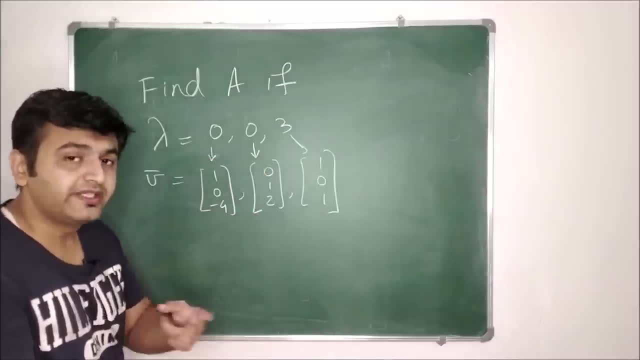 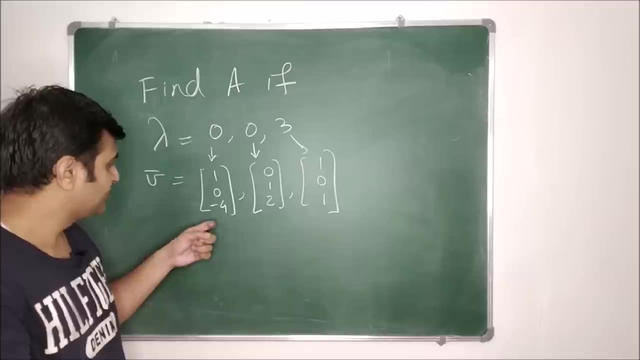 So for that I should have GM to be 2. that means I should have two linearly independent eigenvectors and you can check that this two are independent. Here there is a 0, here there is a 0. that means you do C1 times this plus C2 times this equal. 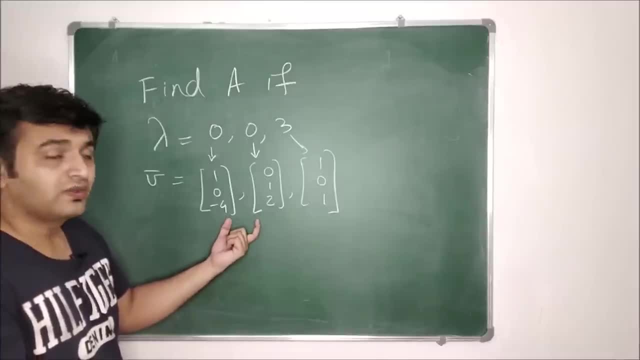 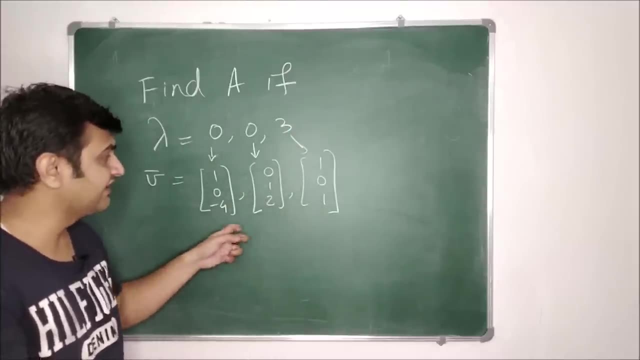 to 0, your C1- C2 will come out to be 0. So these two eigenvectors are linearly independent eigenvectors for eigenvalue 0 and this is independent for this. So overall, these three vectors are linearly independent. and now your job is to find the 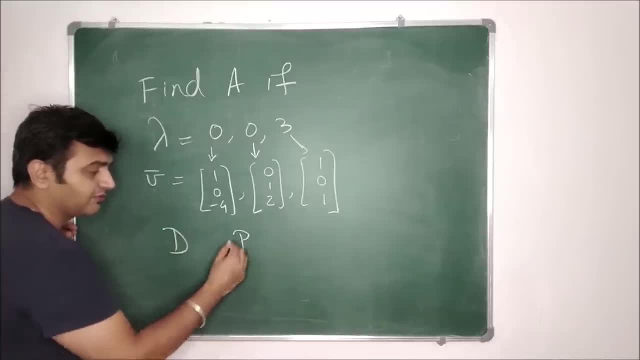 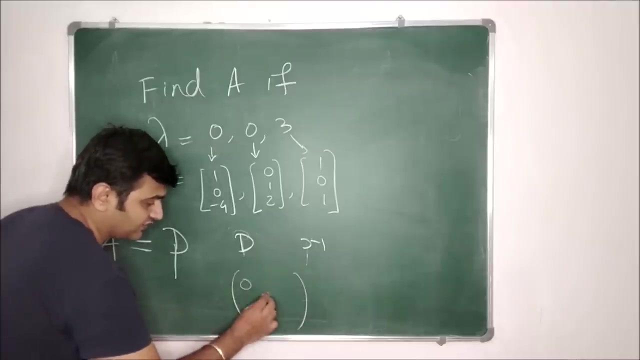 matrix A. So write down the matrix D, Write down the matrix A, Write down the matrix P. Find the matrix P inverse and do this multiplication, PDP inverse. you get the answer A. The only thing one has to be cautious is if you are writing 0, 0, 3.